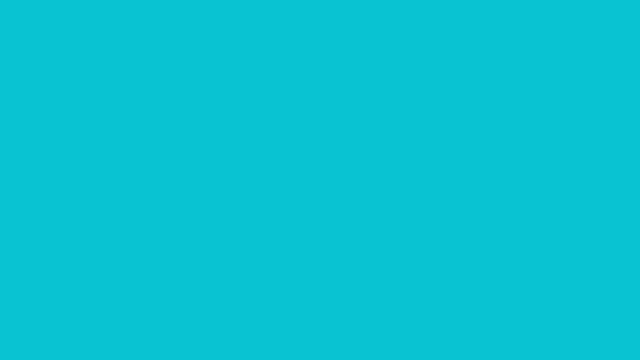 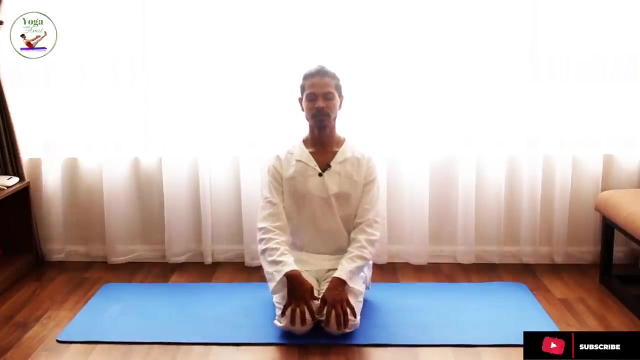 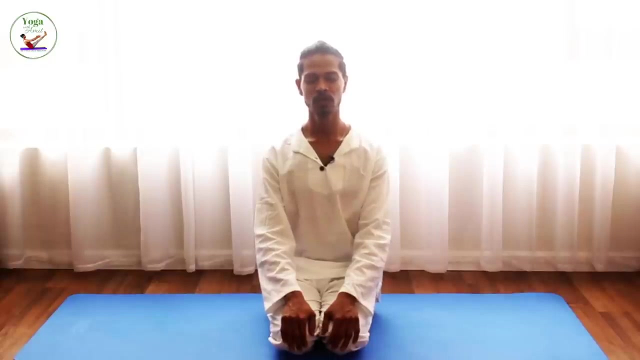 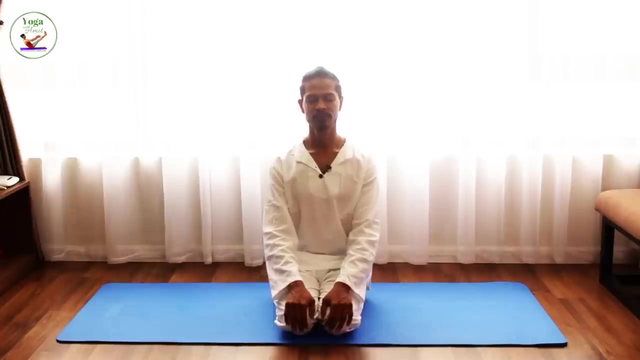 First of all, sit in Vajrasana and bring your hands onto your knees. Keep your eyes closed. Let Vajrasana, the most powerful pose, work for your healing to start When you see the Vajrasana exist on your worked surface. 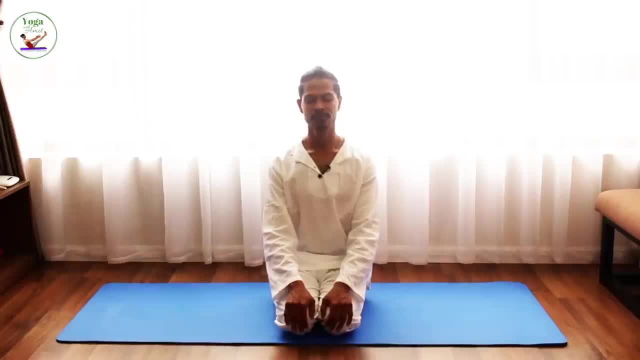 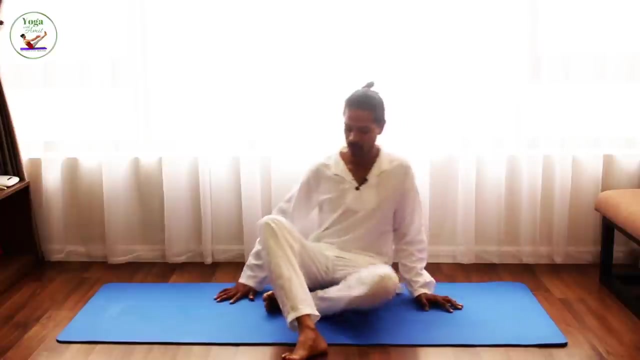 When you see the Vajrasana, you can hear the sound of candlelight flashing light in the dark. First of all, focus on your practice, on the things you want to do, And gently open your eyes and bring your feet out and join the sole of the feet together. 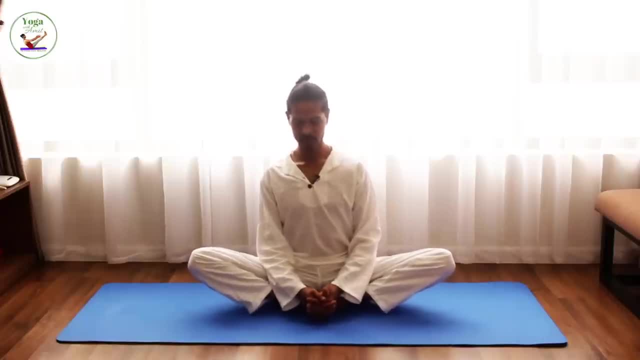 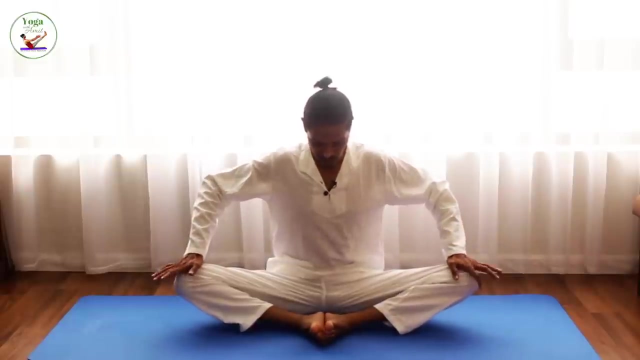 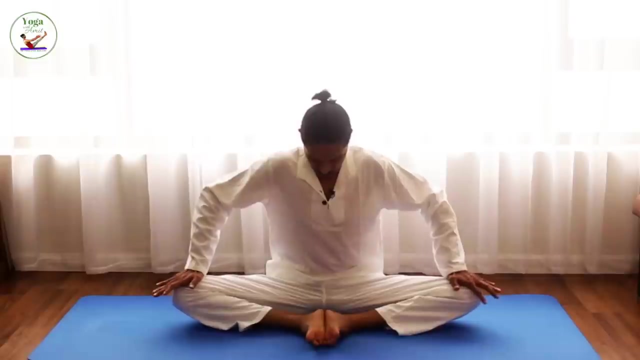 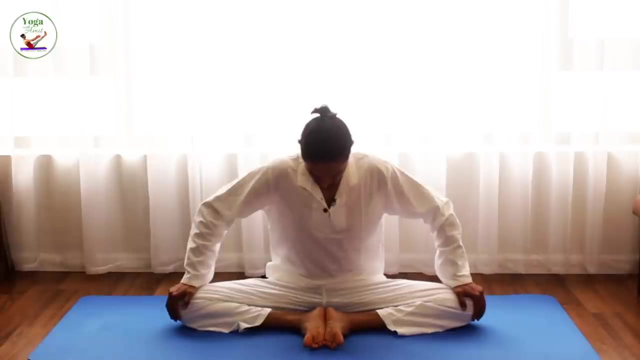 Lift your chest up, close your eyes, shake your legs and gradually stop. Bring your feet slightly forward. Hands on the knees: I'm giving pressure to your knees as much as you can, Keeping your back straight. If your knee doesn't touch the ground, it's okay. 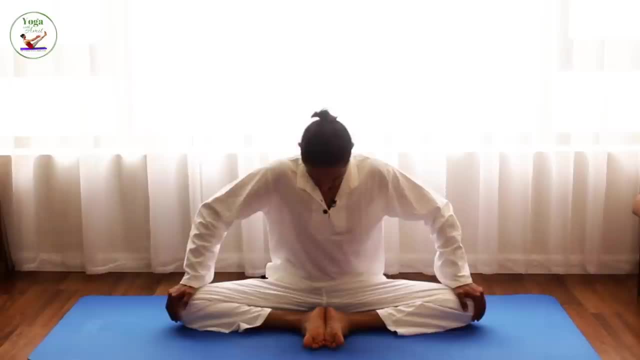 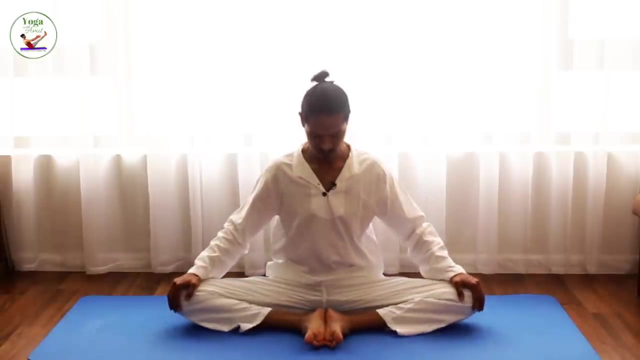 And gently movable your left foot. Stop And gently come back up, Stretch your legs out. Hey, really So do you want to be able to do some? you know incredible movements of your body that you're used to like recherching that stuff. 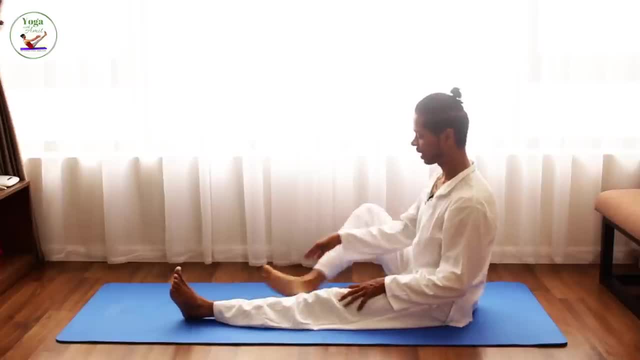 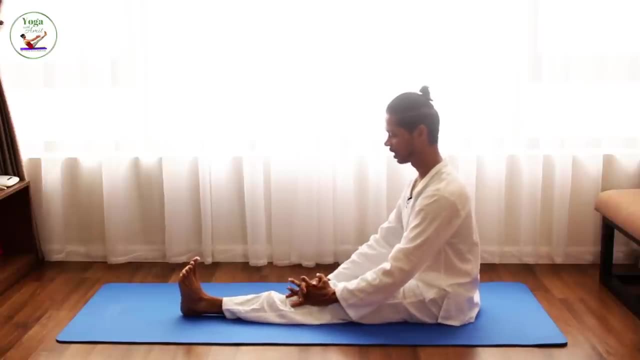 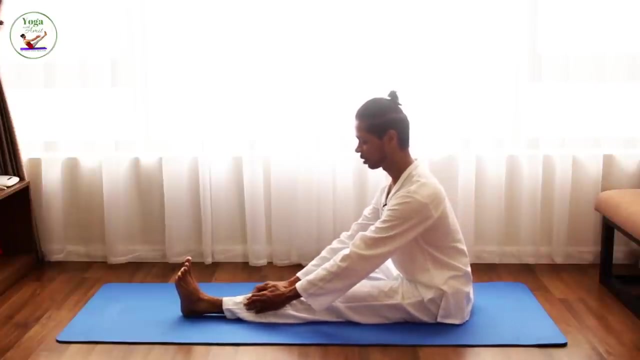 Yeah, yeah, sure, OK, so we're able to do seven pussy Paintings. and bend your right leg close to your perineum, hands onto your knee, inhale, lift your chest up and, with exhale, each exhale, go forward. as you exhale, bend. 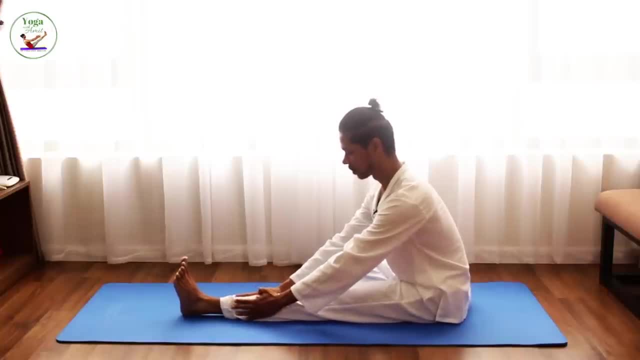 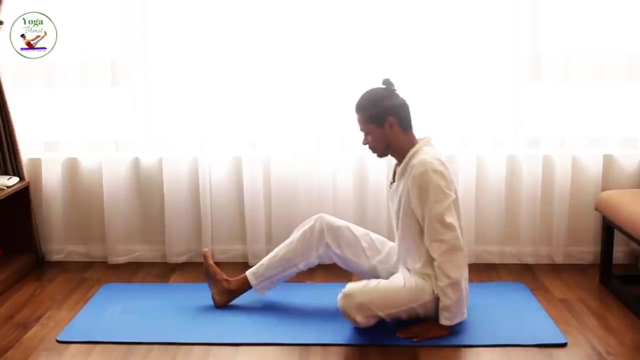 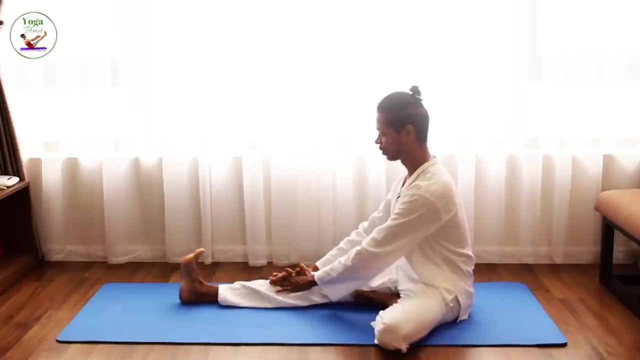 forward slightly more, keeping your back straight, foot active, bringing your toes towards your face and heel out, keeping the breathing normal. the next inhalation: bringing your hands forward, up and down, changing the neck, stretching right leg hands onto your knee or shin bones, lift chest up as you. 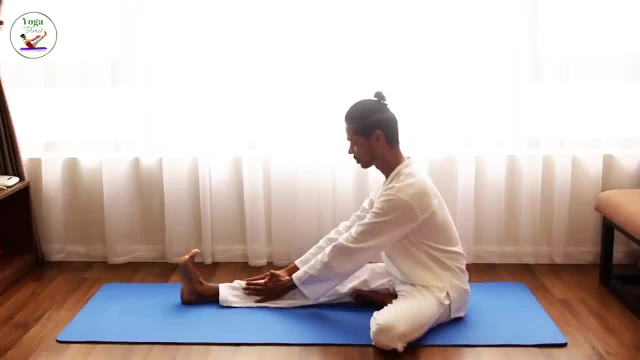 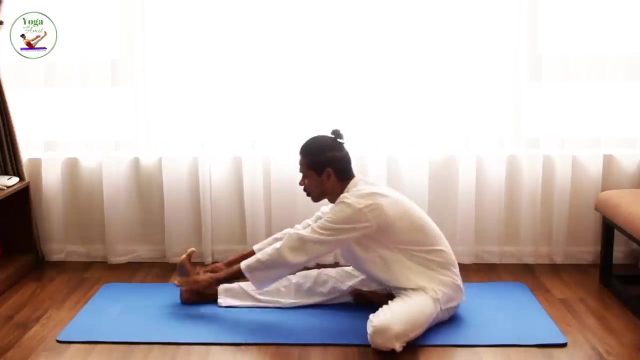 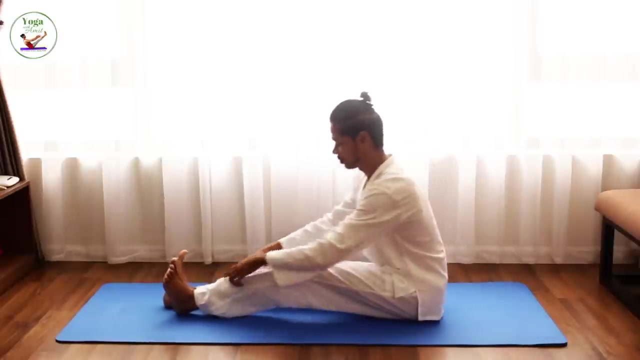 inhale with exhale. bend forward a little bit more forward. stay there, you. the next den variation, bringing your hands out, up and down. the next den variation: bringing your hands out up and down and down. stretch both legs out, repeating the same with both legs, at the same time lifting your chest. 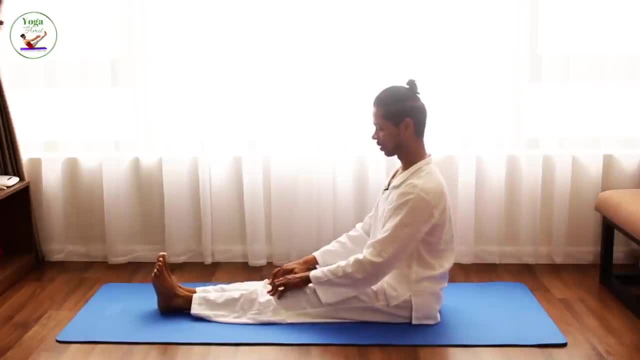 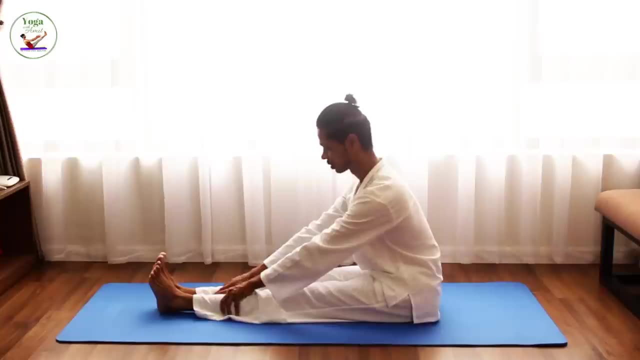 up keeping your hands onto your leg and, as you exhale, bending forward slightly more forward, and stay there. if you can try going each and if you can try going each, and if you can try going each with your exhale forward slightly forward, with your exhale forward slightly forward. 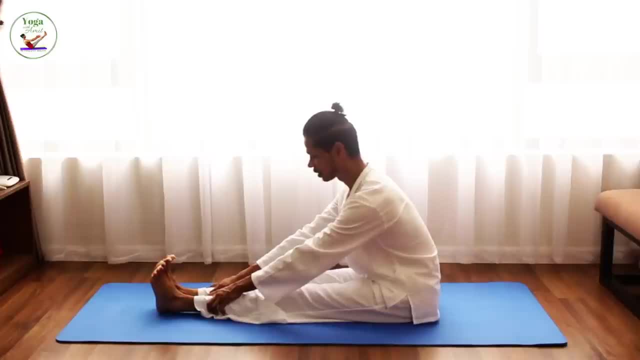 with your exhale forward, slightly forward. you want to make sure, you want to make sure, you want to make sure that your back remains straight on the next inhalation, bringing your on the next inhalation, bringing your on the next inhalation, bringing your arms forward, arms forward. 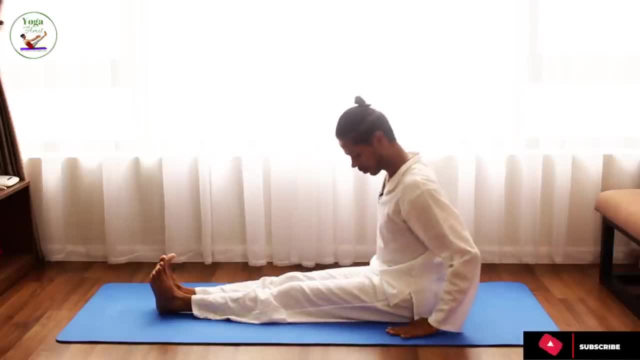 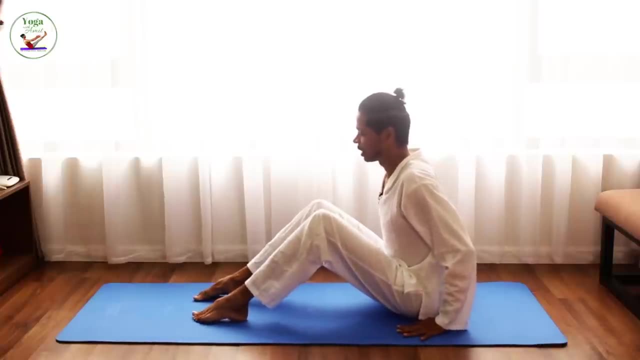 arms forward, up and down, up and down, up and down. bring your hands by the side of the body. bring your hands by the side of the body. bring your hands by the side of the body. bend your knees wide open and inhale. bend your knees wide open and inhale. 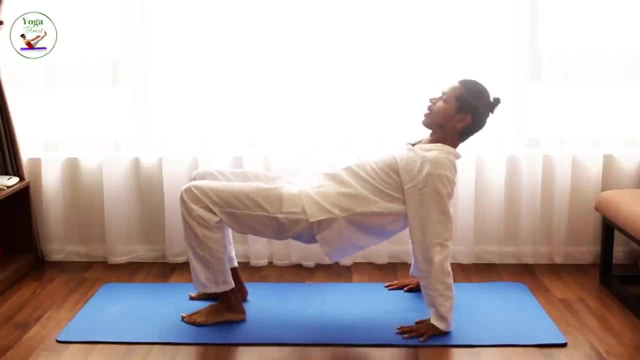 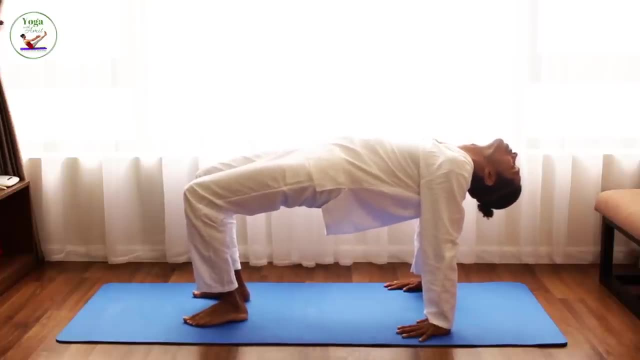 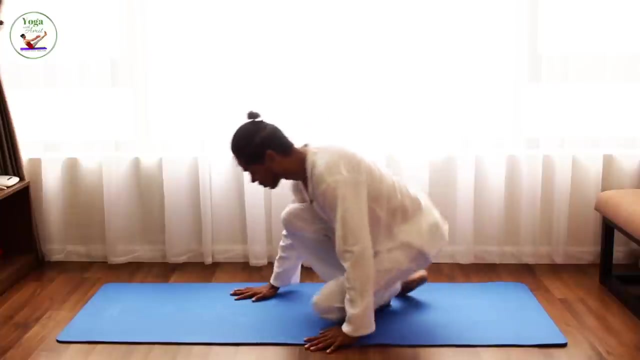 bend your knees wide open and inhale, lifting your hips all the way up head, lifting your hips all the way up head, lifting your hips all the way up head, back, back, back, back back, exhale down, exhale down, exhale down and lie on your abdomen. 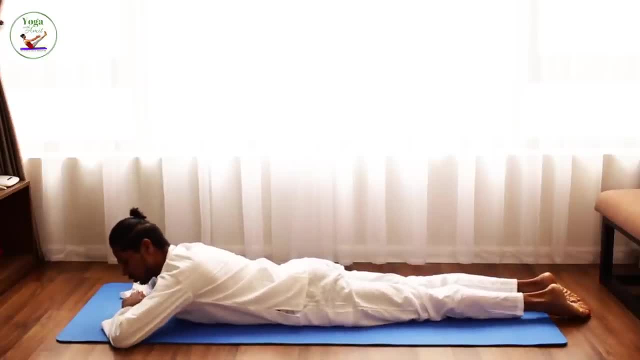 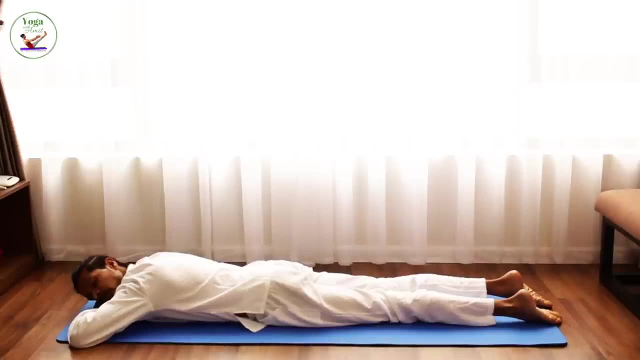 and lie on your abdomen. and lie on your abdomen, bring your hands on top of each other. bring your hands on top of each other. bring your hands on top of each other. relaxing, relaxing, relaxing. face onto your hand, face onto your hand, face onto your hand, giving a gentle massage to your lower. 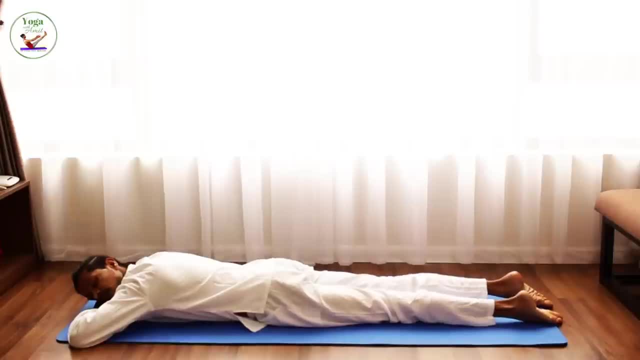 giving a gentle massage to your lower, giving a gentle massage to your lower abdomen, abdomen, abdomen and inhale. lift your head up and inhale. lift your head up and inhale. lift your head up. turn your face to the other side. turn your face to the other side. 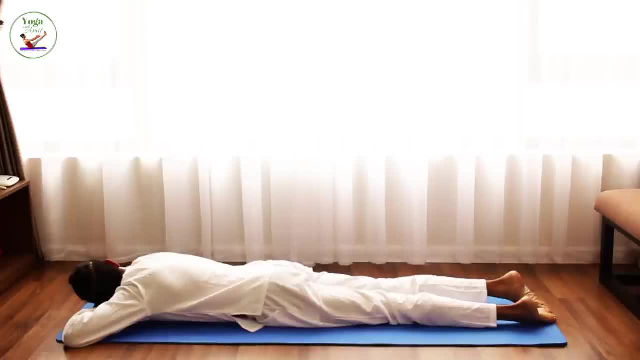 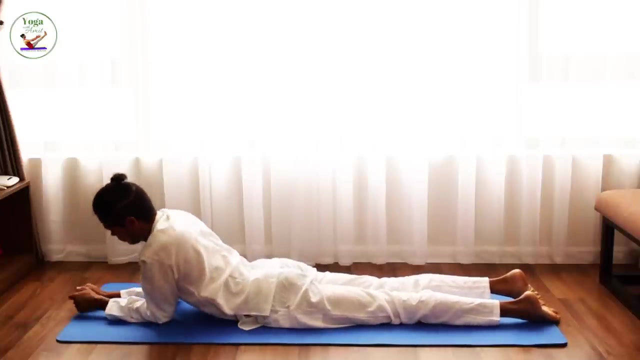 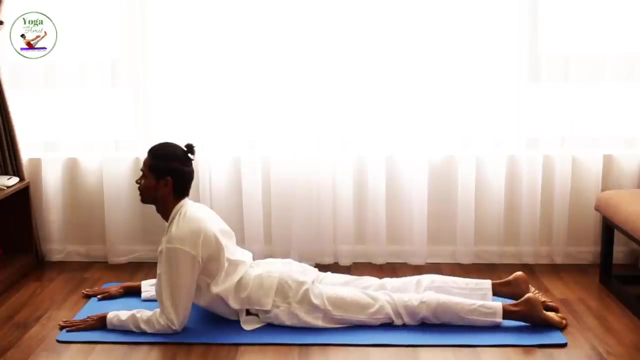 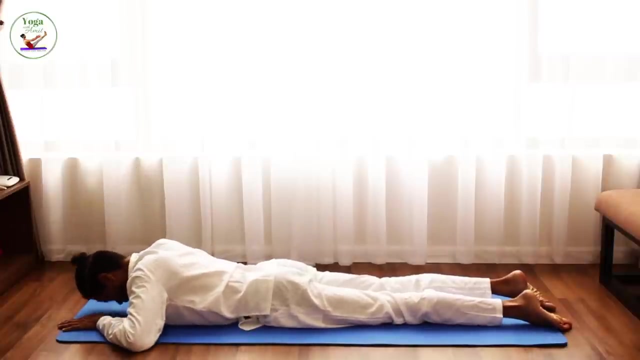 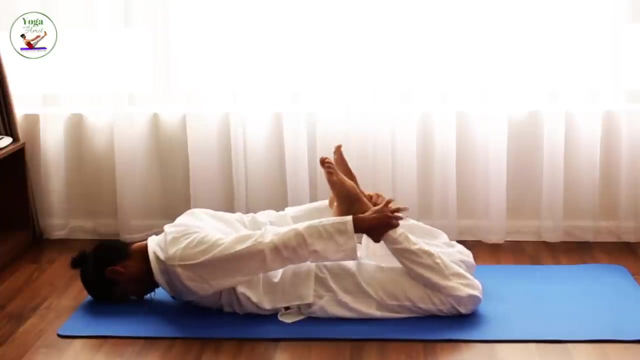 Thank you. Then very slowly coming up, standing on the elbows, palm about, shoulder-wide apart, lift your chest up, shoulder down, look forward, Keep your breathing normal, Exhale down, bring your forehead on the ground, bend your knees, hold your ankles, then inhale. 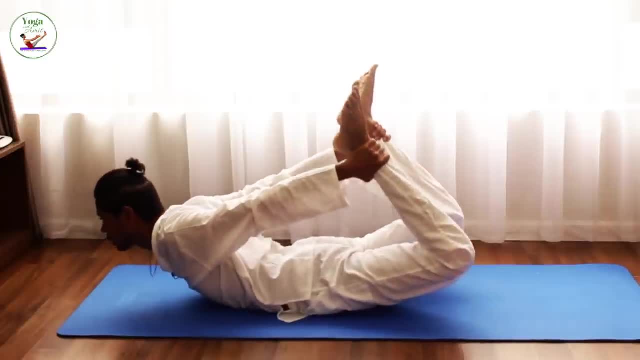 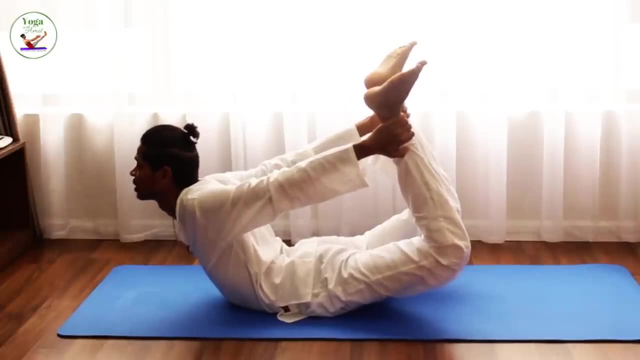 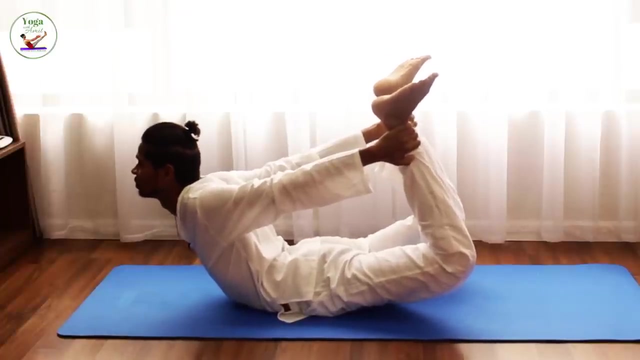 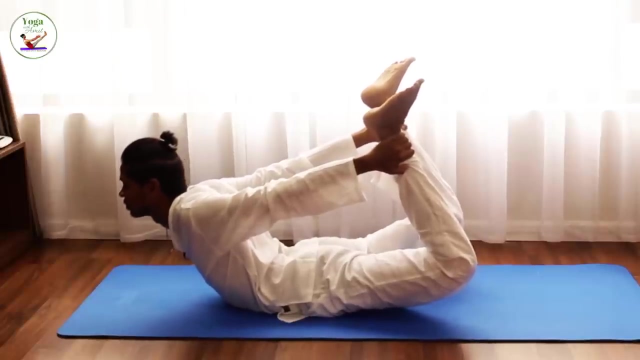 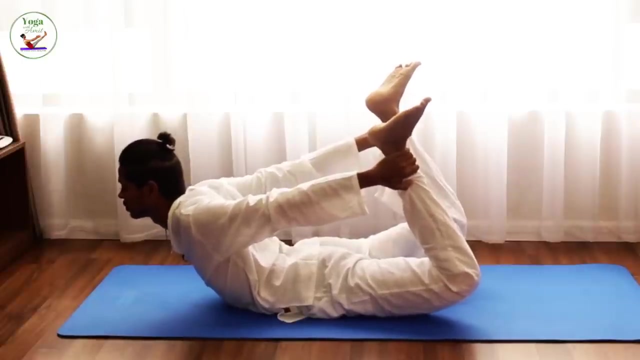 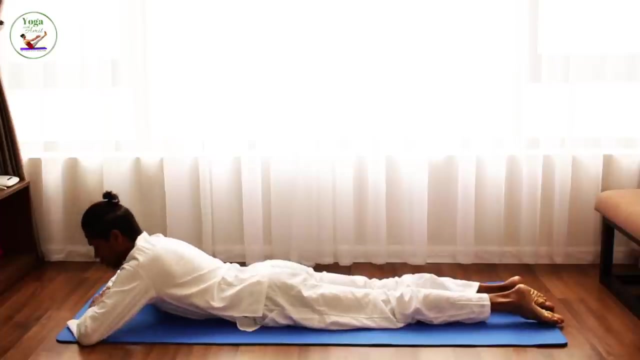 lifting your head up, shoulders up, chest up, arching your back, All giving Such by breathing in and out long and deep. Come down and go back into Makrasana, your hands on top of each other And face relaxing on the head. 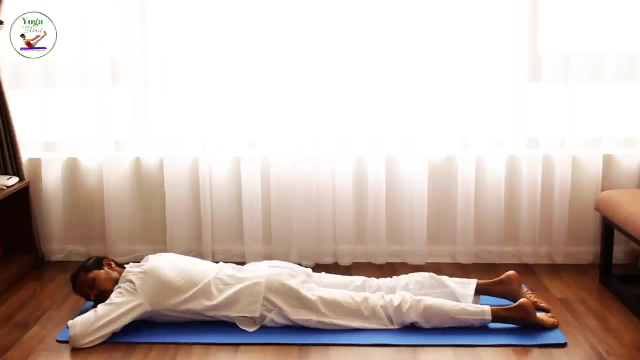 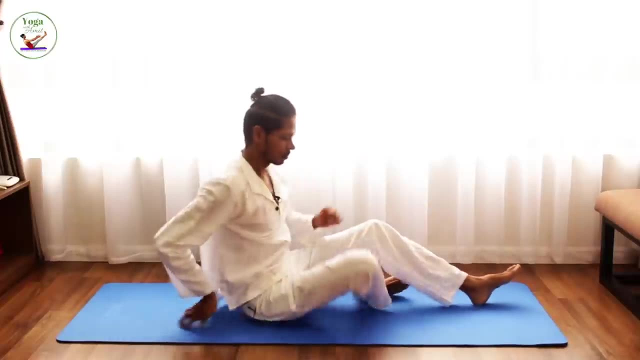 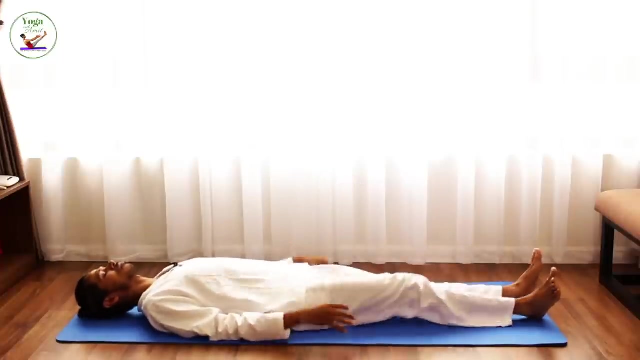 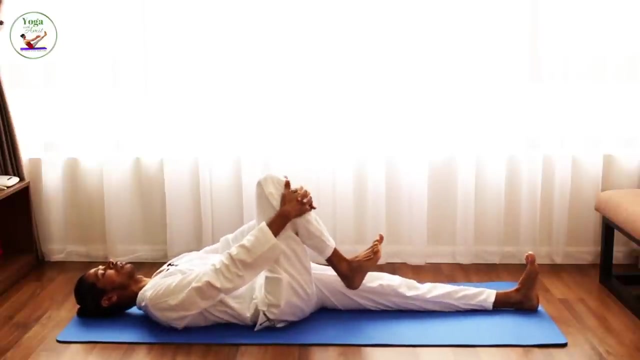 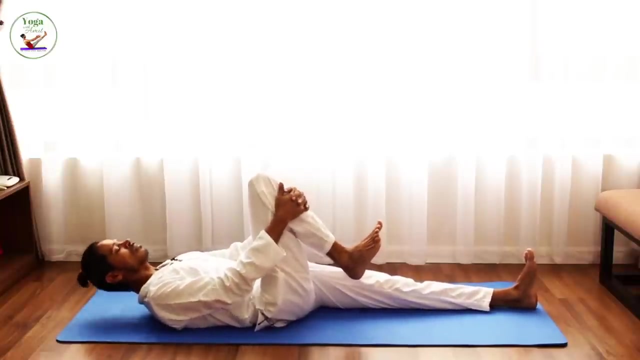 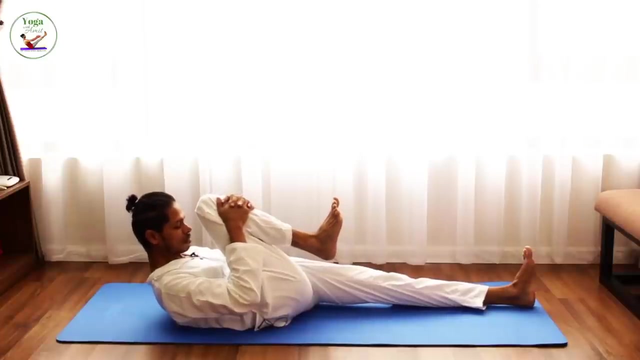 And gently push with your hands, lie on to the back And bending your right knee, grabbing with your hands. Inhale, lift your head, touch your forehead to the knee. Exhale, lift up your arm, pearls back and close your eyes. 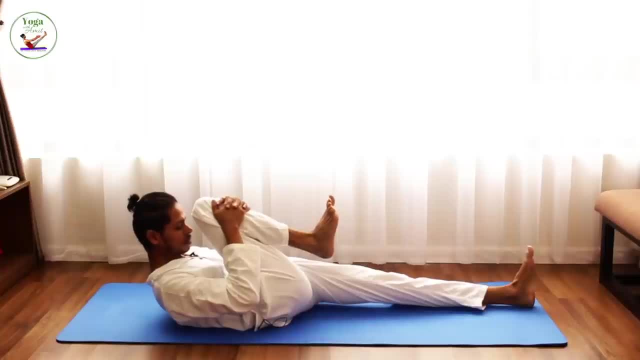 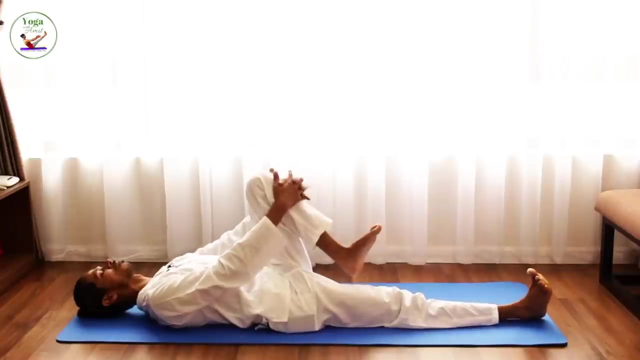 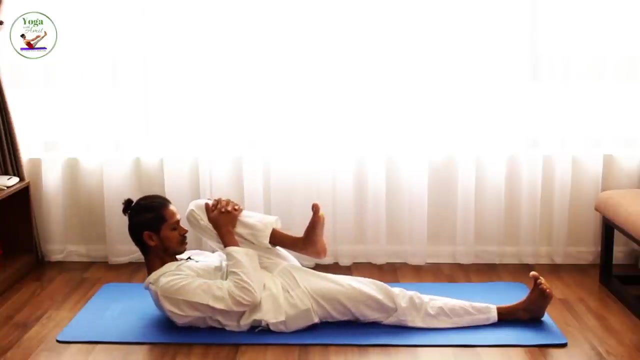 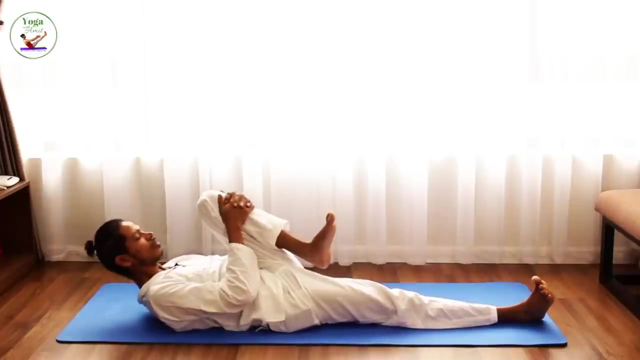 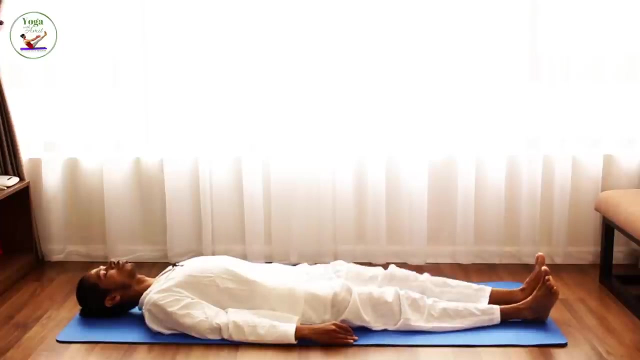 Seal it down into linear petal pose, exhale down. repeat the same on the other side, bending the left knee, grabbing your leg with your hands. inhale, exhale. bring your head to the knee, exhale down. extend your legs out. and now we will repeat the same with both. 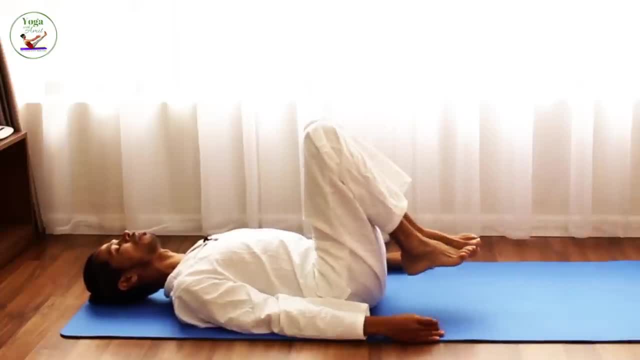 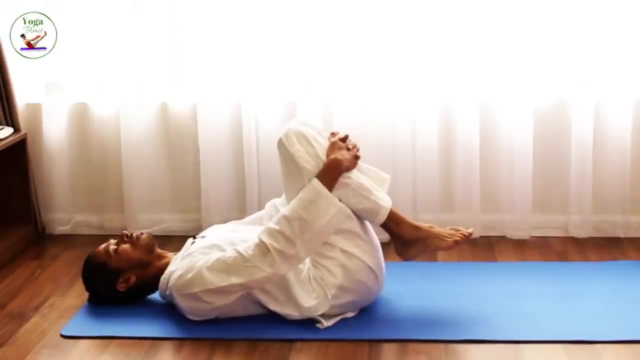 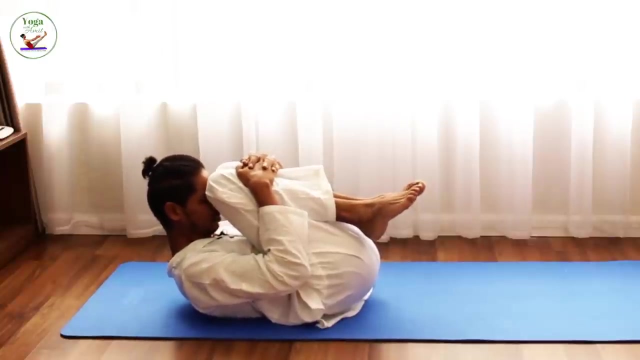 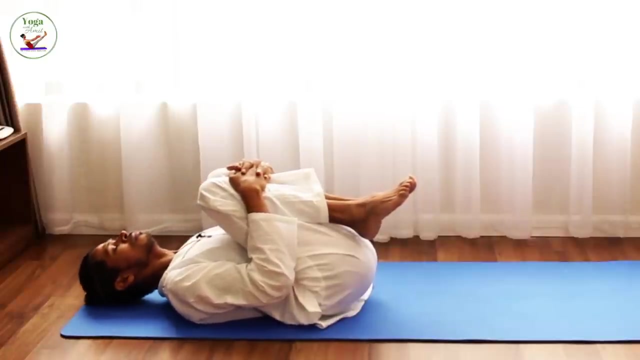 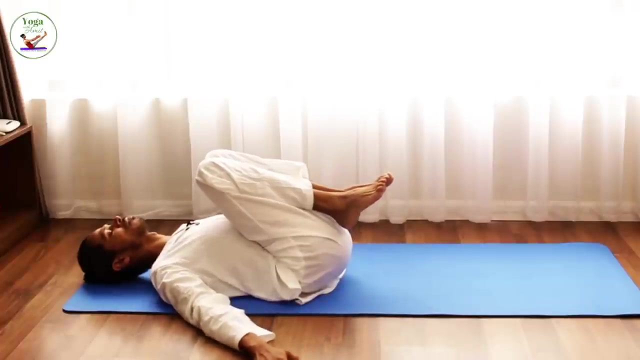 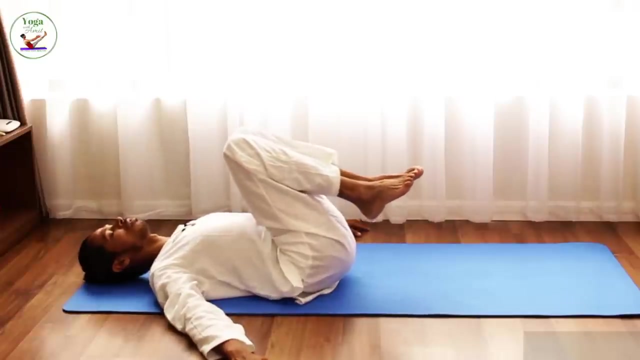 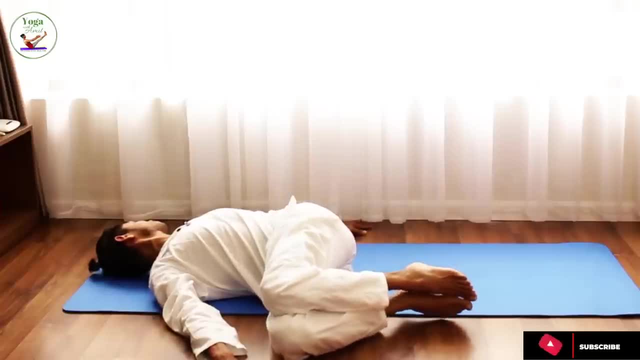 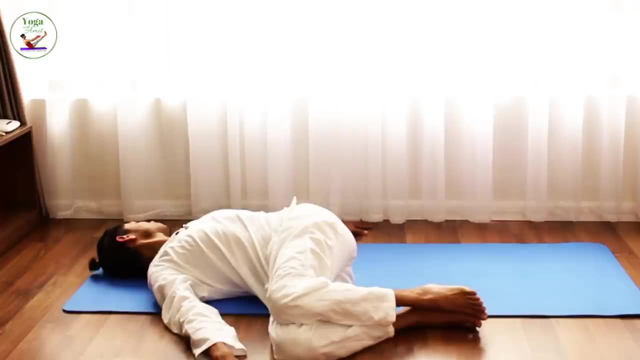 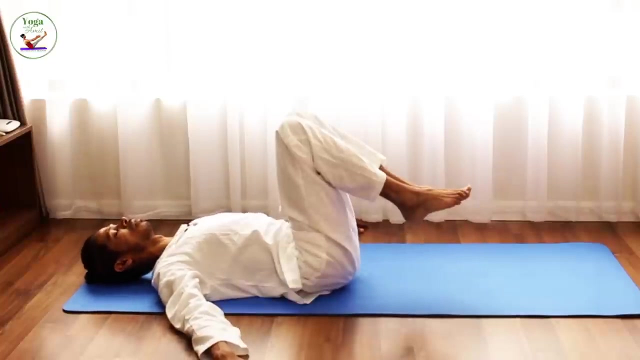 look to the left. bring your legs back down. bring your legs back down. bring your legs back to the center. bring your legs back down as you exhale. drop them to the left. look to the right as you exhale. drop them to the left. look to the right. 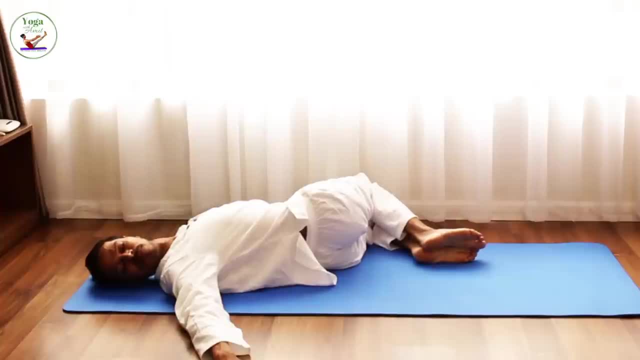 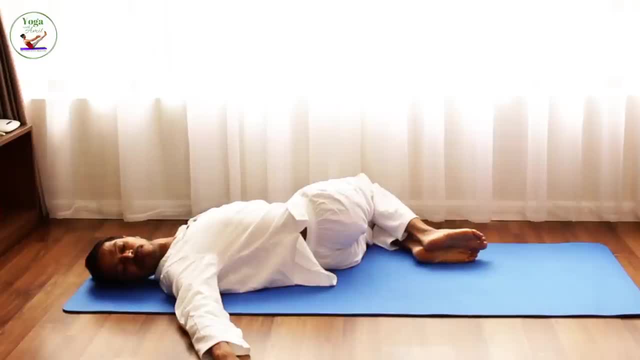 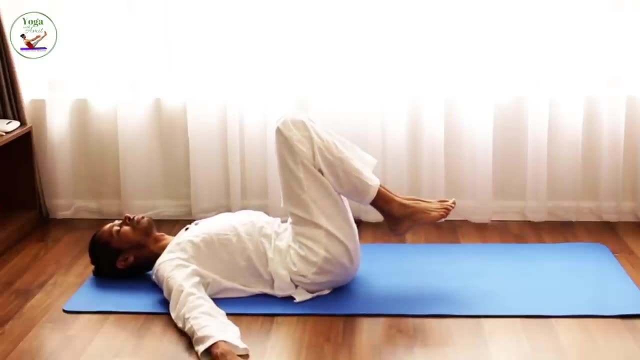 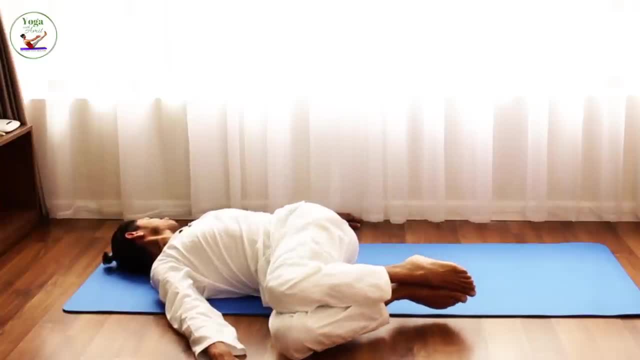 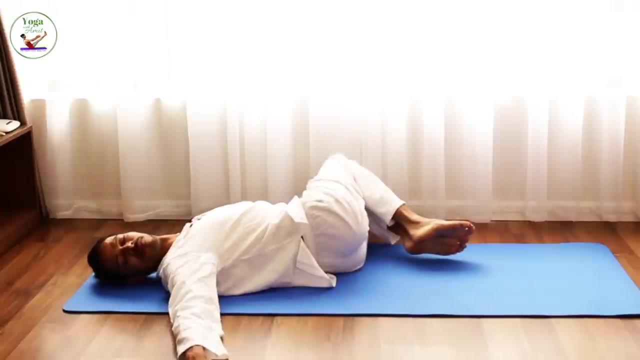 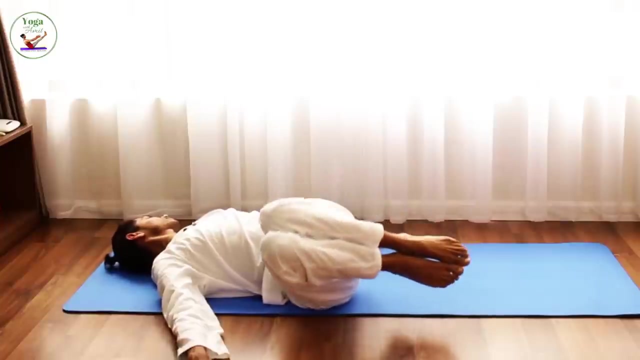 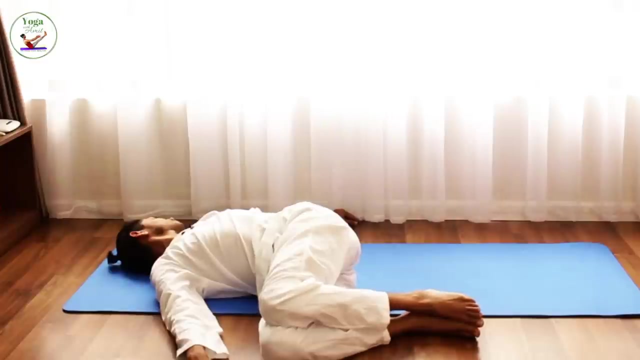 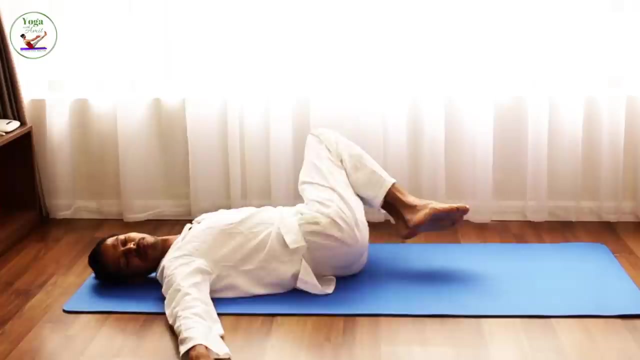 to the center. let's repeat two times each side: Back to the center, to the left. To the center, to the right. To the center. to the left. To the center. to the right, To the center, to the left. 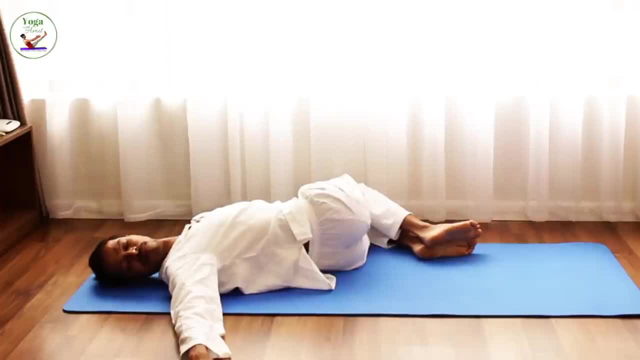 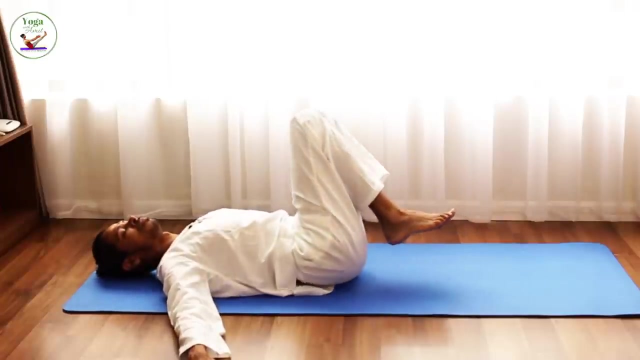 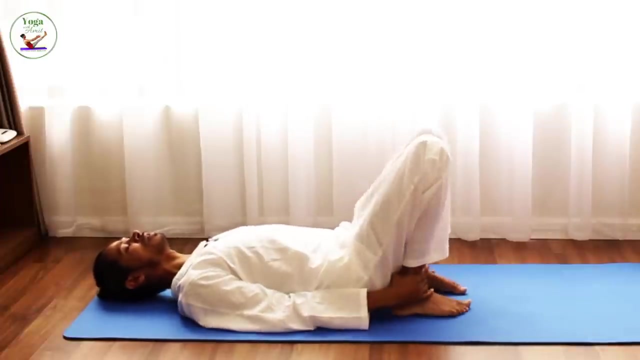 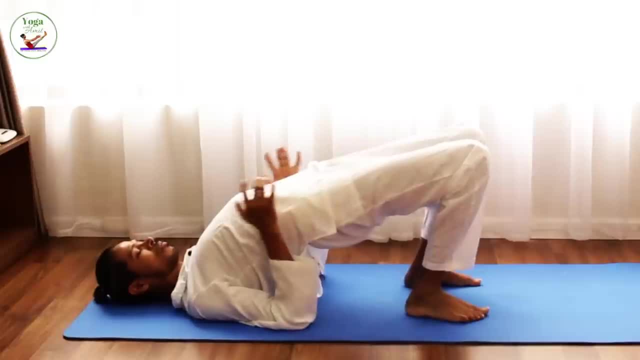 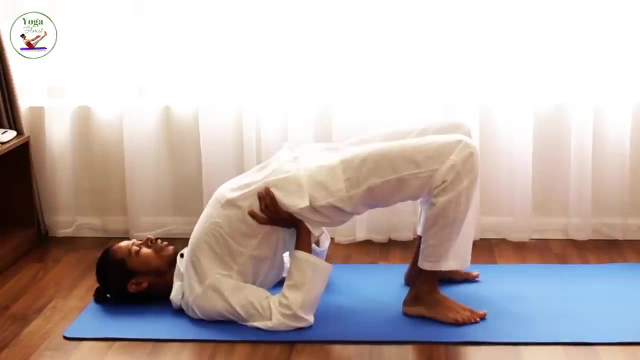 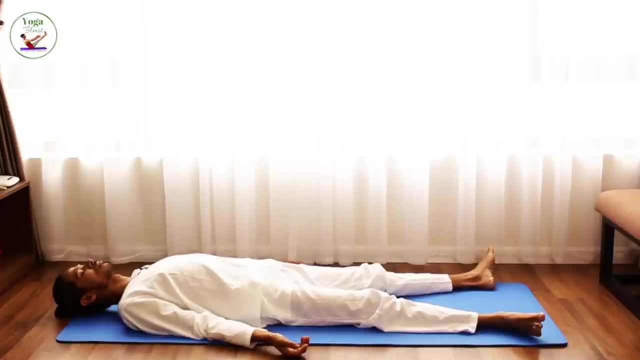 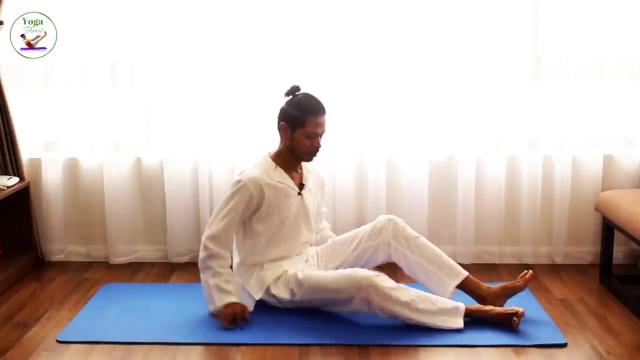 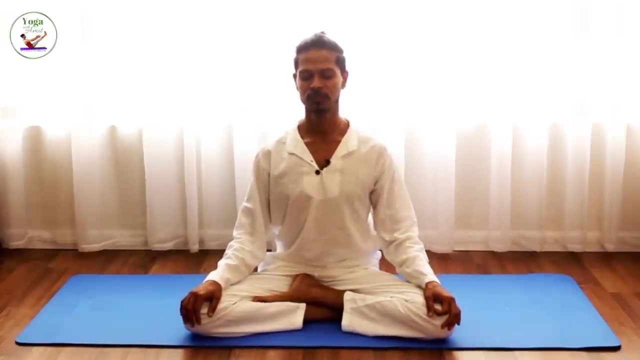 To get health, To get health, To get health. Thank you, Thank you, Thank you. Then gently turn to your right, Push with your hands, Sit up, Sit quietly for a while And become aware how this practice made you more calm. 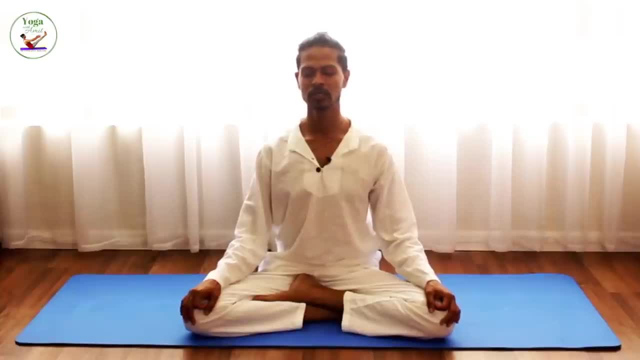 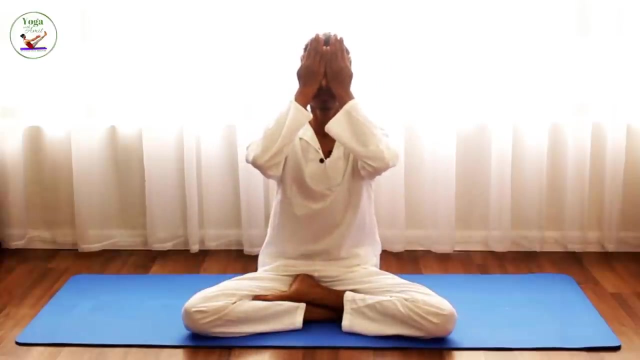 or relaxed, And the healing comes. Gently rub your palm together, Bring your hands onto your eyes, onto your face. Rub your face One more time, Rub your palm together And bring them onto your lower abdomen. Give some warmth and the healing